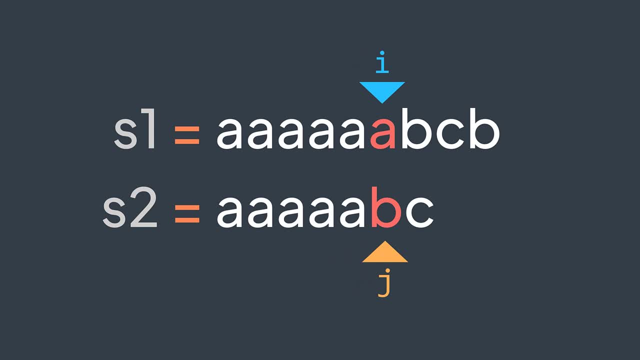 where we started. Why didn't we just continue from the actual index I? We would avoid losing time on always going back in s1.. Take some seconds to think about it. It's true that when we started from the first index of s1, it didn't match s2, we 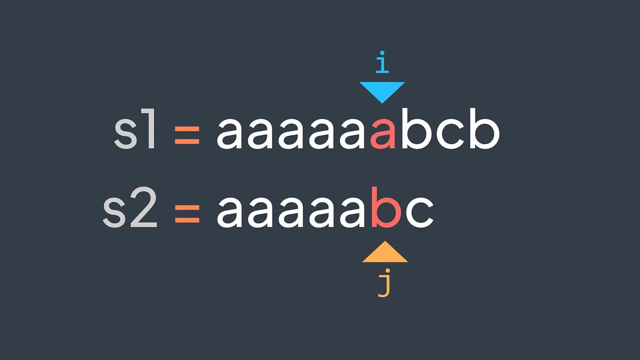 found a mismatch at index five. Now we need to start searching again. But if we decide to start from the actual index, we may miss a prefix that would lead us to the match we're searching for. For example, if we just start from, I will have a match. then we have b and 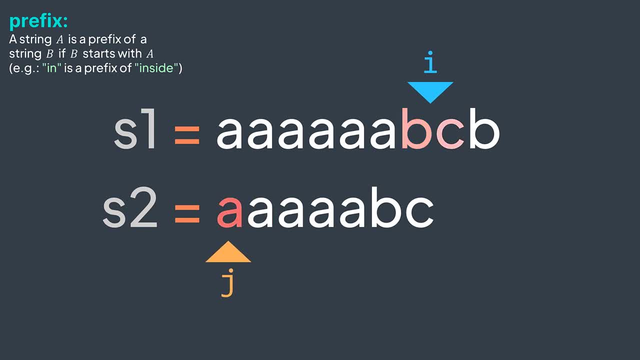 a mismatch. We'll start again. b and a mismatch. We'll start from the next index c and a mismatch. We start from the next index b and a mismatch. And we finished traversing s1 without finding s2, we would say that s2 is not present in s1. It's because 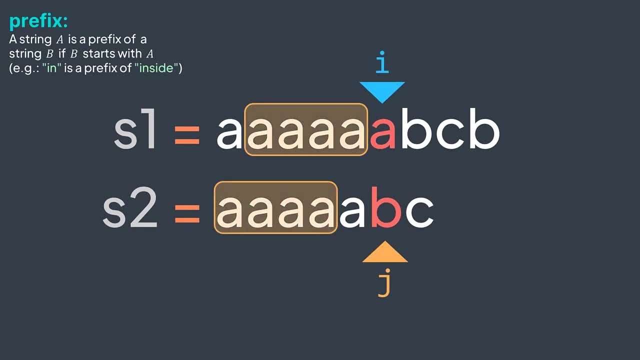 we skipped an important prefix of s2, which is a a a a. You can see that at the mismatch position we already matched with a a a and if we just continue from after a, a a, we have a match, then b match, then c match and we finished as two. 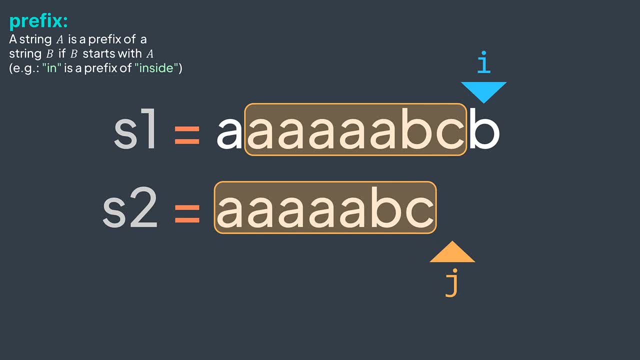 And this is why in the brute force solution we always go back from where we started and we move to the next index to start from there, to avoid skipping important prefixes that we already matched with before. But always going back is kind of slow. we need to optimize it. 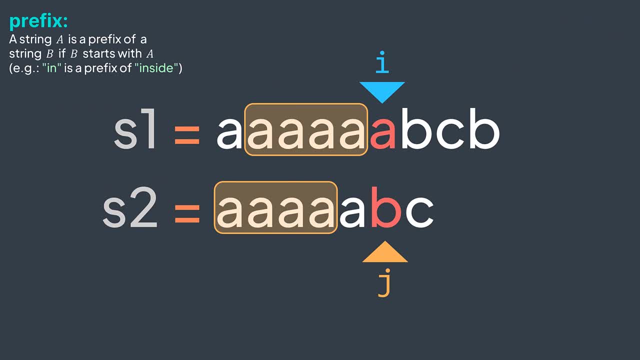 In the last example, when we found a mismatch, we could notice that we already matched with a a a a before. This is why we didn't take I back. we just started after a a a in s2. And we could continue matching. knowing that we matched with a a is what gave us the ability. 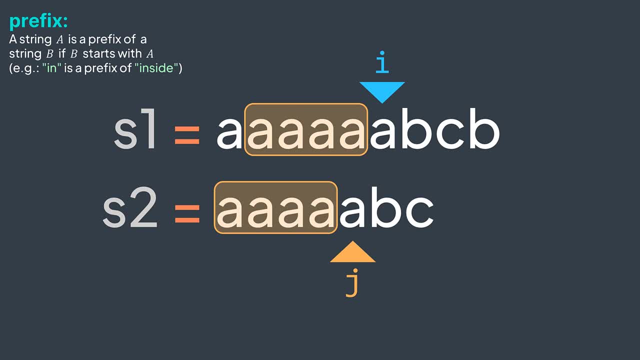 to avoid losing time and going back on s1 and traversing and got the same characters. So the idea is that, instead of taking I back to where we started, we just check what prefix we already traversed and start again from it, For example in this situation: okay, 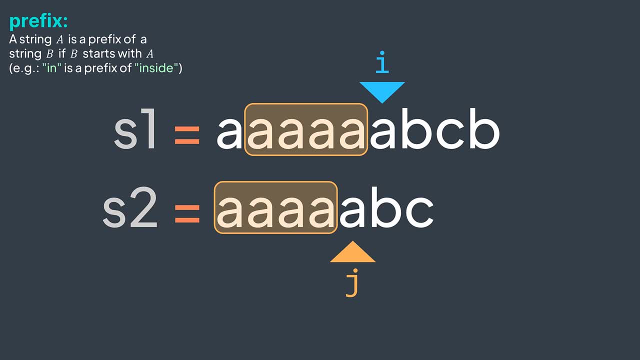 there is a mismatch, but to already matched with a a a, we'll start from index four and s2, because the length of a a a is four. But the question is why AAA and not another one? First of all, AAA is not the only prefix. 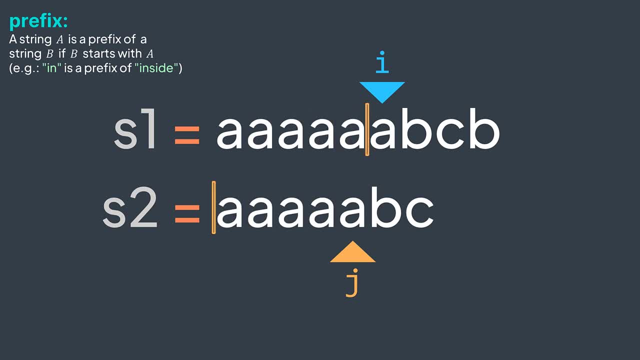 we also have AAA, AAA and the empty string. We took AAA because it's the longest proper prefix. we take the longest one because we want to avoid traversing again as much characters as possible. I said longest proper prefix. What does proper prefix mean? A proper prefix? 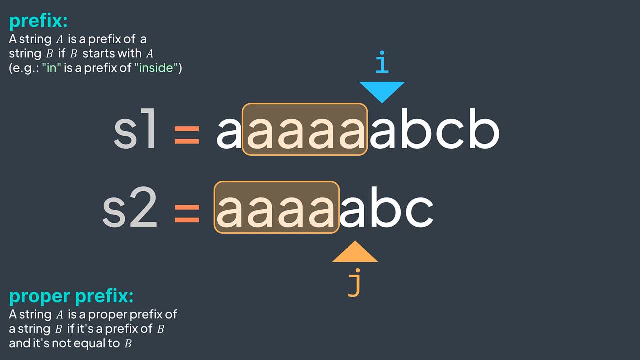 of a string. s is a prefix of s. that is different from s is true that s is a prefix of itself, but it's not considered as a proper prefix. The proper prefixes of s are prefixes of s minus s. We take the longest proper prefix because in reality, the longest one is the 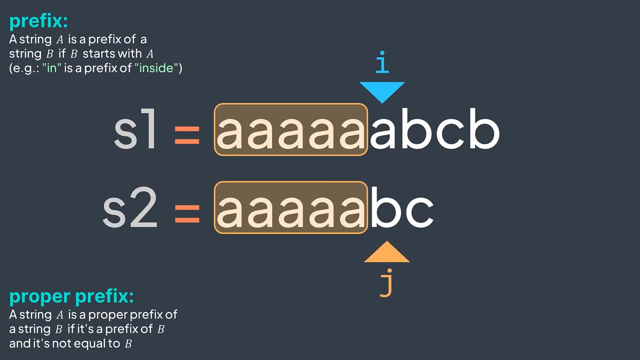 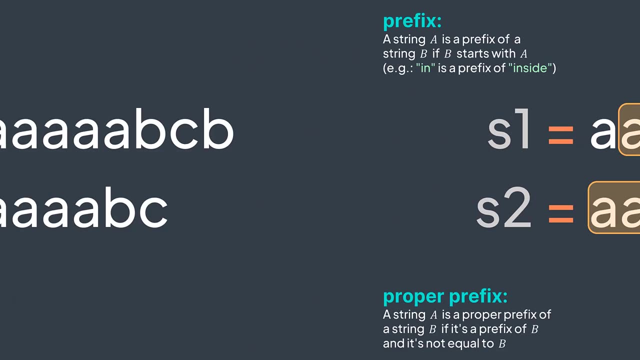 whole string itself, the part we already matched. And if we take it, we know that it won't lead us to the match researching for because we found a mismatch. This is why we take the longest proper prefix. Next question: How did we know that it's AAA and not something else? We started from the first index and 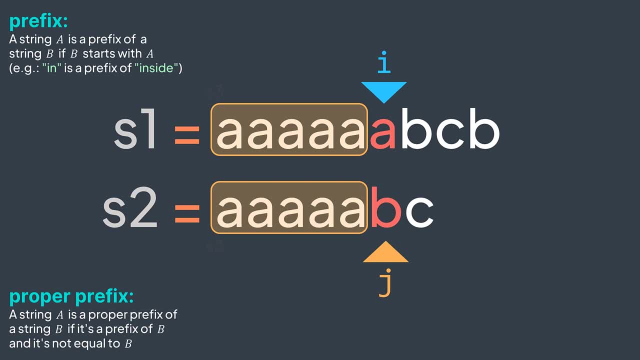 we matched with the part AAA. Then we found a mismatch. Let's name the part that matched as three. We're searching for proper prefix of s, three. that is as long as possible, But don't forget that it has to also be a suffix of s3 and s1, because we will continue from. 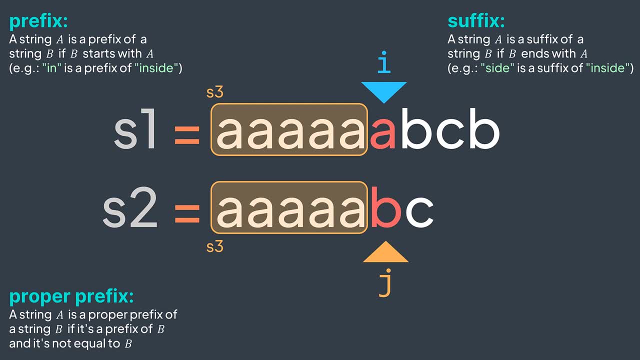 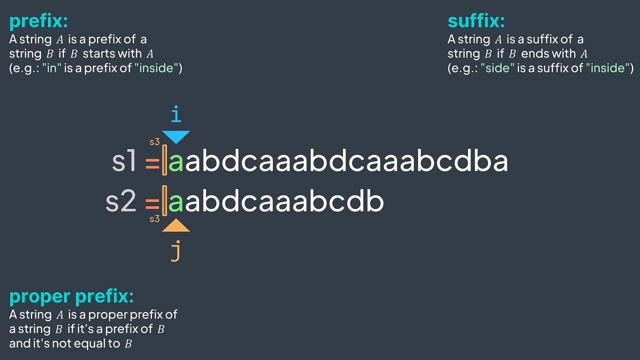 the right and characters must be adjacent. In brief, we need to search for the longest proper prefix of s2.. So let's take a look at the suffix of s3. that is also a suffix In our example. it's AAA. It's not that clear with this example. Let's take this one. We start from the first index. 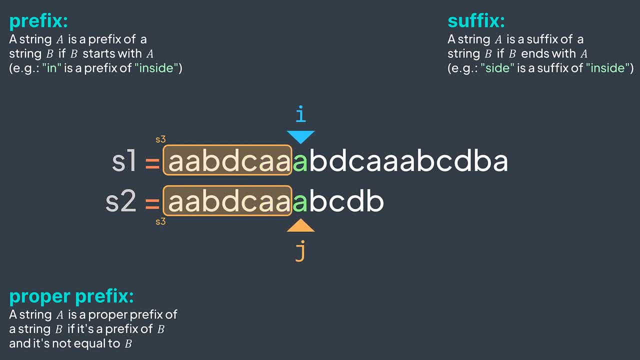 we have a a, b, d, c, a a a b, then mismatch Here the longest proper prefix that is also a suffix of s3 that we traversed before, is a a b. by traverse before I mean that answer the end of s3, s1, to be able to continue taking characters. 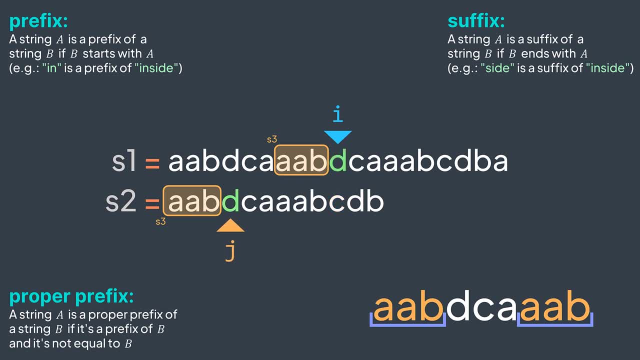 We take J to the position just after it in s2.. Then we take D, c, a, a, a, B, C, D, d and we found s2 and s1. You can see that we took the longest proper prefix. that is also a suffix of s3, we skipped its characters to avoid losing time and we continued matching without. 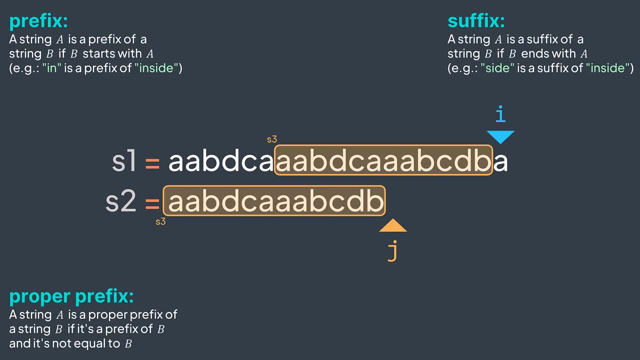 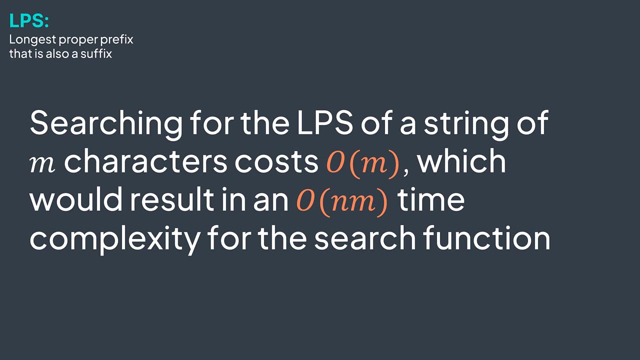 taking. I back In brief. when we find the mismatch, we search for the length of the longest proper prefix. that is also a suffix of the part that matched, to know how many characters to skip again. But searching for the longest proper prefix, that is also a suffix of a string of M characters. 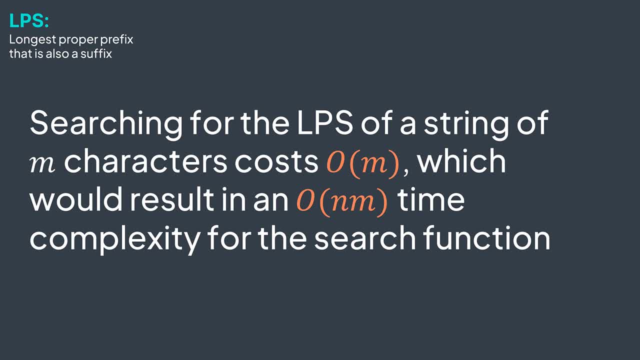 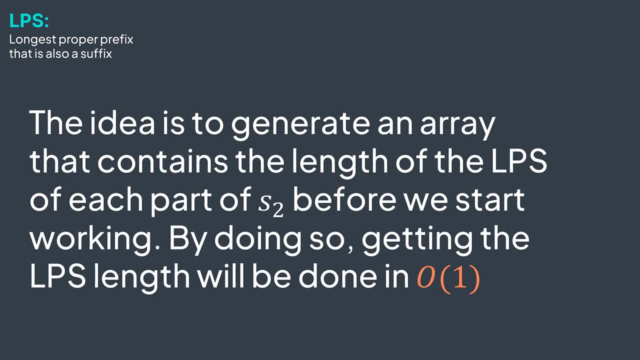 costs of m time And by doing it at each iteration we would get the O of m times m time complexity again. it's like we did nothing. But what if, instead of always losing of m time to compute the length of the LPS, we compute the length of the LPS for each part of s2 at. 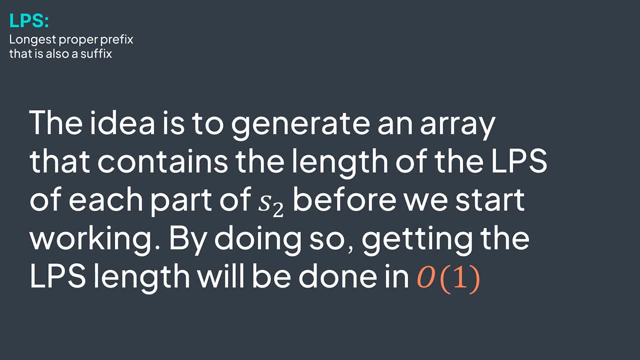 the beginning. we put the results in an array so that when we start working, finding the length of the LPS will cost of one only. we just take the value from the array, And that's what the KMP algorithm does. It starts by doing some pre processing to create the LPS array- an array. 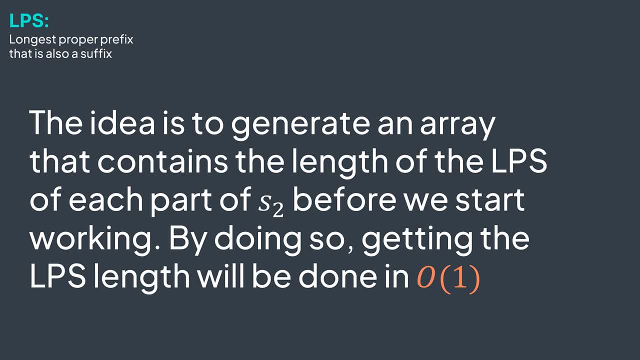 where LPS of k represents the length of the longest proper prefix. that is also a suffix of the first k plus one characters of s2, then it starts working on s1.. For example, if s2 is equal to the string in LPS array, we'd get 01012223.. 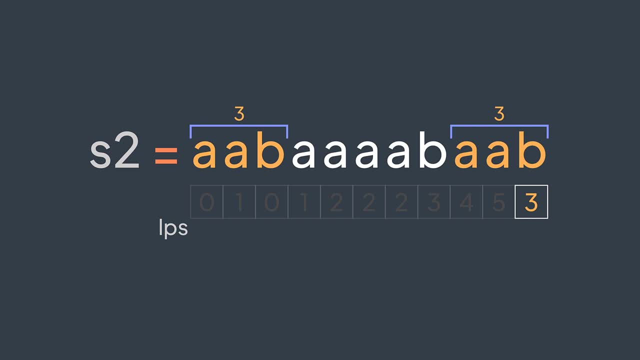 But how to actually compute these values. that's what we will see. now We have a brute force solution for finding the length of the LPS for each part, But we want to have an optimized solution. we will try to do it in of m time only. 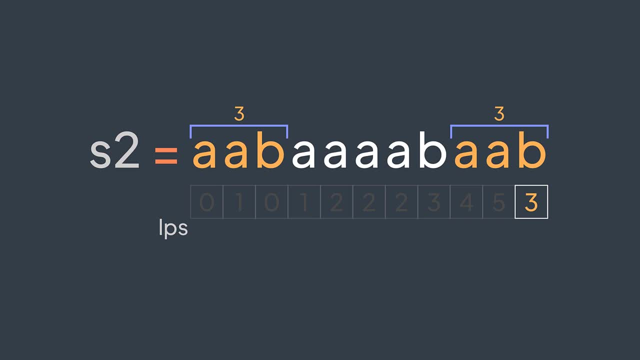 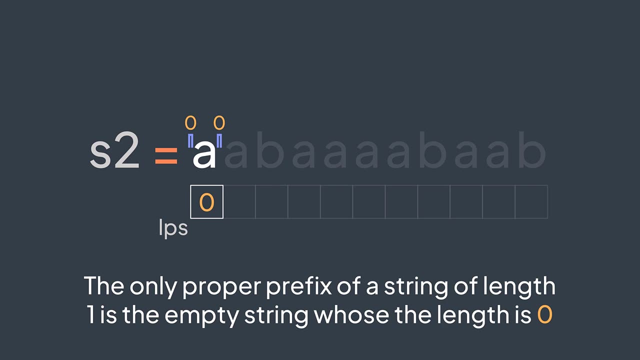 not more. We'll create an array of m elements and we start when we have one character only. the only proper prefix is the empty string is length is zero, So LPS of zero will all always be zero. And now the idea to fill remaining cells is that if we know the LPS of the first k, 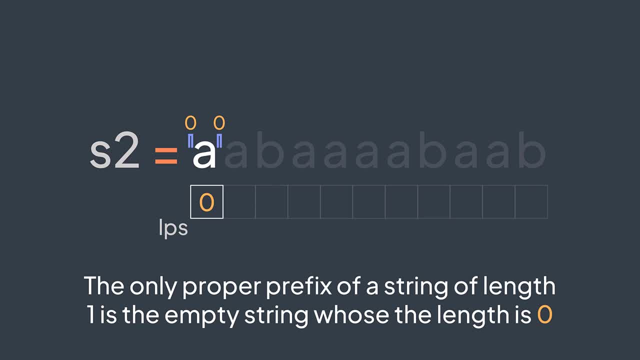 characters and we want to know the LPS of the first k plus one characters. we compare the character k plus one with the character just after the LPS. So we will use the LPS of the first k characters to find the LPS of the first k plus one characters. For example, if we have this string: 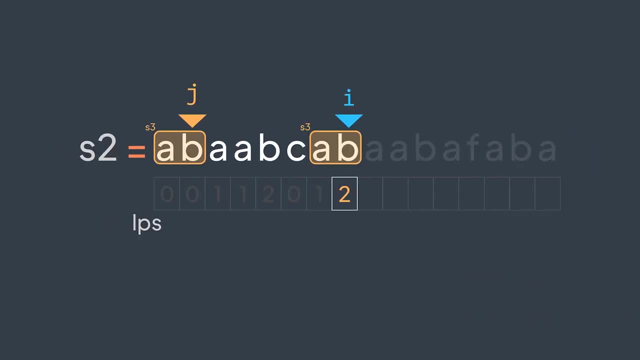 and we're at this position. the LPS is a B. Now if we want the LPS of the part that has one position in it, we increment both i and j and we compare here: s of i and s of j are equal, so we can extend. 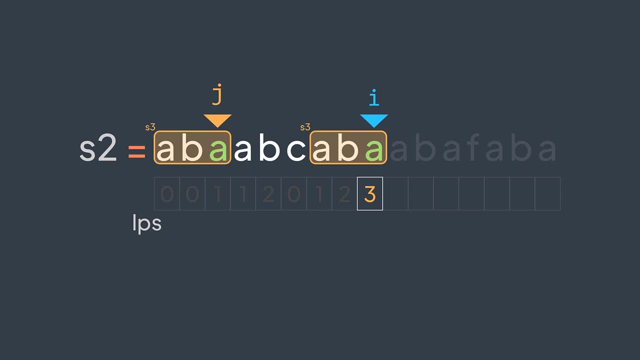 the LPS of the previous position. the LPS of this position is a, b, a. next iteration, after incrementing i and j. here s of i and s of j are also equal. we extend: the LCS of this position is a, b, a, a. next iteration: same thing. we extend the LCS of this position is a, b, a, b. next iteration: here they: 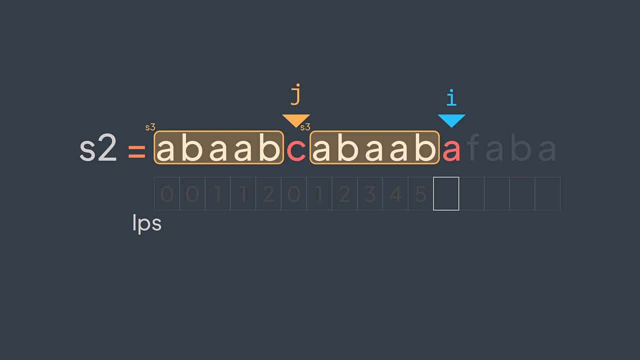 we cannot extend But we don't start again from the beginning- which are the LPS of the part that matched Here. the part that matches a, b, a a b. the length of its LPS is two. we could know it from the array by checking the cell j minus one of the LPS array, which is two. 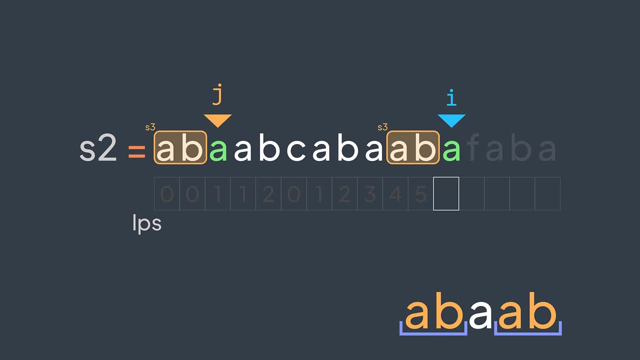 so we take j to two. Know that we have no problem to find the LPS of the part that matters because we already computed it. Now. s of i and s of j match. we can extend. the LPS is a ba. Next iteration: s of i and s of j don't match. we check the LPS of the part that matched. 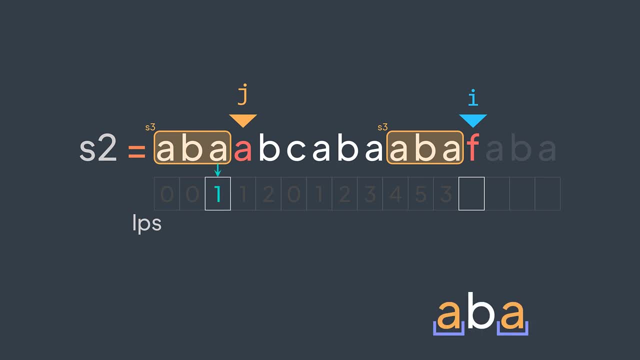 the part that matches a, b, a, the length of its LPS is one we take j to one s of i and s of j don't match. and the part that matches a, its LPS, is the empty string. the length is zero. 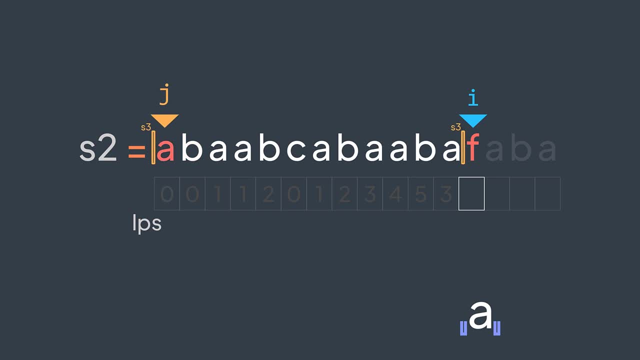 we take j to zero. s of i and s of j don't match, And here j is zero. It means that we just don't have a proper prefix suffix except the empty string for the part that ends at I would just put math i to start again from the next position. Then here, as of i and s of j match, we extend. 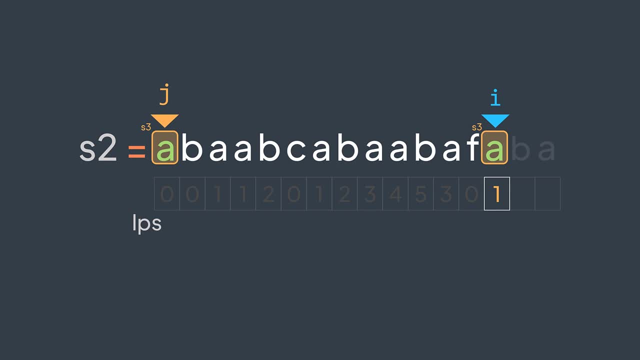 the LPS is a will put one and will continue like that until we finish traversing the string from this example. we didn't use that. at each iteration we compare s of i and s of j and we have three cases: the case where they match, the case where they don't match And Jason greater than zero and the 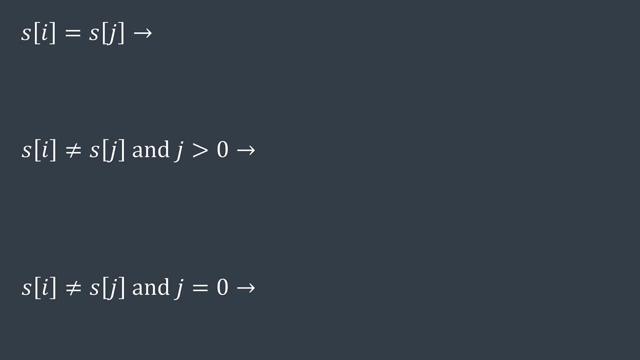 case where they match, where they don't match and j is greater than zero, And the case where they don't match and j zero. when they match, we can extend. we increment j, which is also the length we put it in LPS of i, and increment i to move to the next cell in the array. 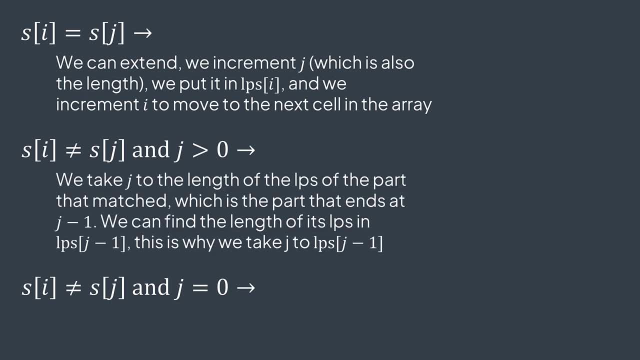 When they don't match and j is greater than zero, we take j to the length of the LPS of the part that matched. and where they don't match and j is equal to zero, we just put zero in LPS of i and increment i to start again from the next position, Because the LPS is the empty string. there is no. 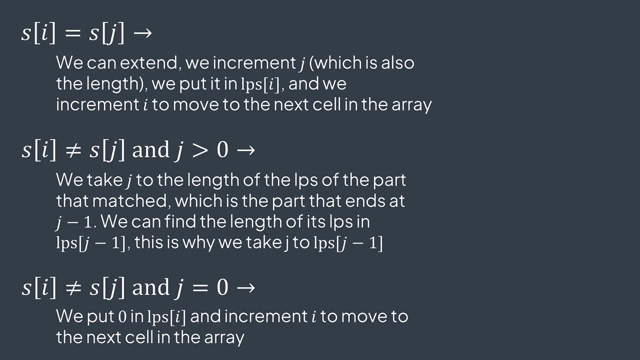 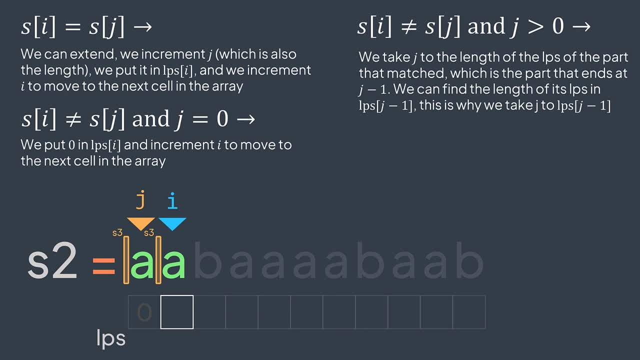 other choice. Let's continue our previous example. now j starts a zero and a at one one, because we already filled LPS of zero. Here they match, So we extend. the LPS is a next iteration. s of i and s of j don't match And the part that matches is a it. LPS is the empty string, the length is zero. we. 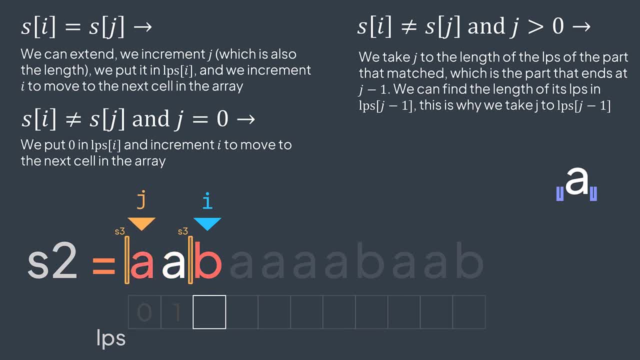 take j to zero. Here again, they don't match and j- zero. we just put zero and move to the next value of i. Here they don't match and j- zero. we just put zero and move to the next value of i Here. they don't match and j zero. we just put zero and move to the next value of i- Here they don't match. Here they don't match and j zero. we just put zero and move to the next value of i. Here they don't match. 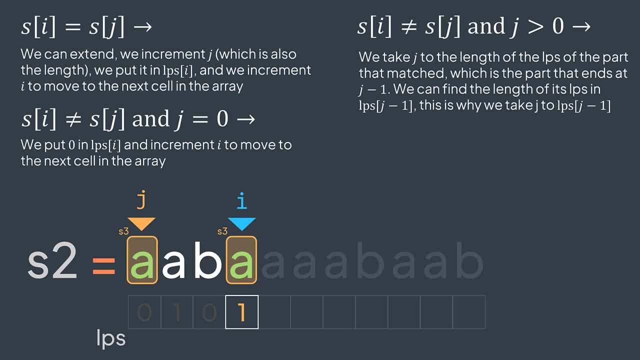 Here they match We extend the LPS is a is length is one. Next iteration: here they match: we extend the LPS is a is length is to next iteration. here they don't match the LPS of the part that matches a length is one. we take j to one. here they match. we extend the LPS is a the length is to next iteration. 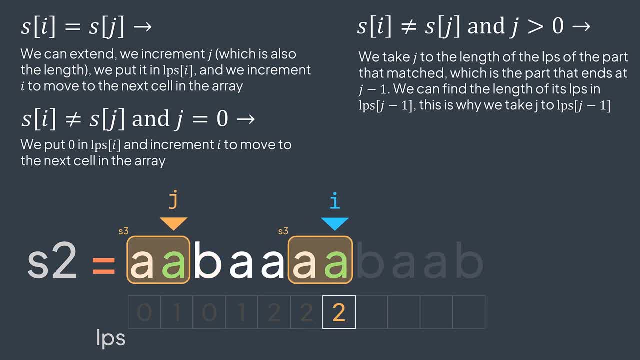 same scenario. j will be taken to one. then they match and we get a as LPS. Next iteration: they match the LPS is a. b length is three. Next iteration: they match the LPS is a. ba length is for next iteration: they match the LPS is a. ba length is five. Next iteration: they don't match an LPS. 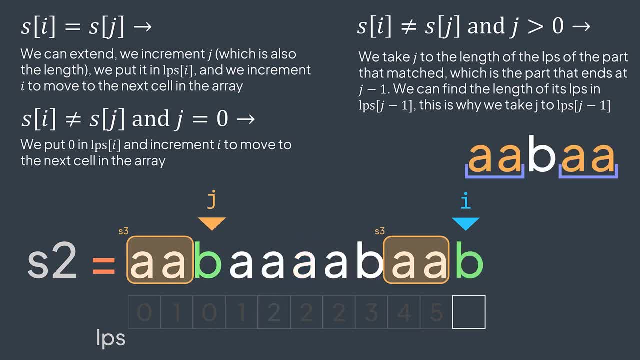 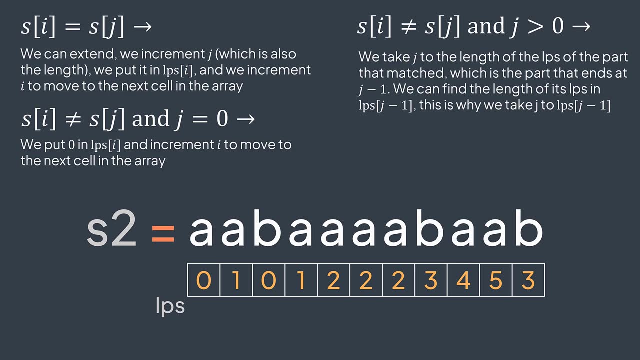 of the part that matches a is, length is two. so we take j to two. Here s of n s of j match we extend the LPS is a, b, we put three. Now I reached the end of s, so if finished filling the LPS array, we return it In code. we create an array LPS of length of s. 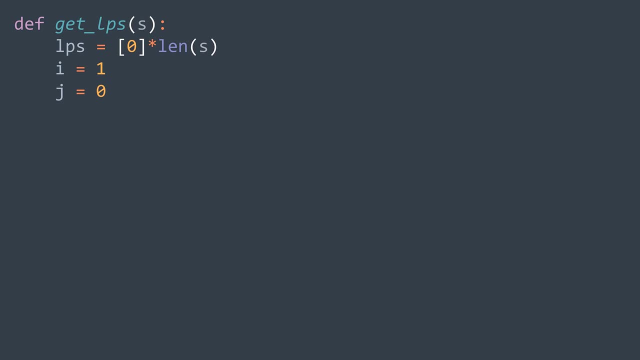 characters who initialize i and j to one and zero respectively. as done earlier, And while I didn't reach the end of the array, we have three cases. If s of i is equal to s of j, then we can extend the length of the LPS is just j- and increment both i and j to move to the next iteration. 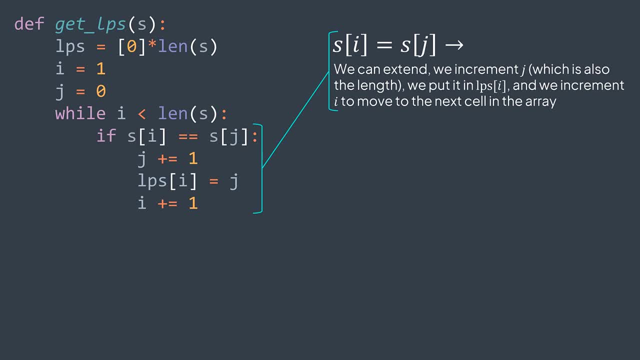 Know that we incremented j before assigning j to LPS of i to get the right length. Second case: they're not equal and j is greater than zero. Here we said that we take j to the length of the LPS of the part that matched. the part that match is in reality the. 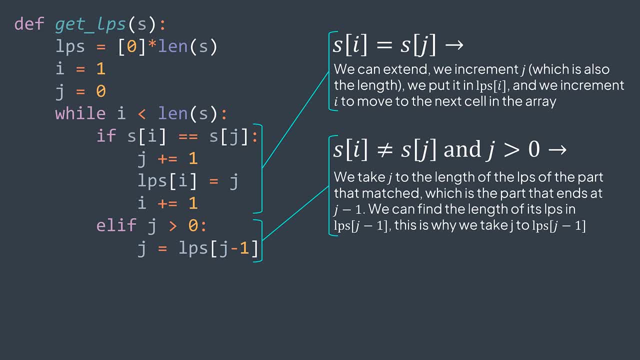 part of s. that answer j minus one, and the length of its LPS is an LPS of j minus one. So j is equal to LPS of j minus one. And last case, when they're not equal and j zero, we just put zero in LPS of i. 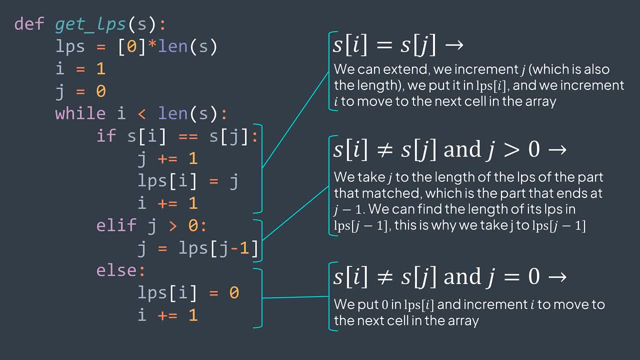 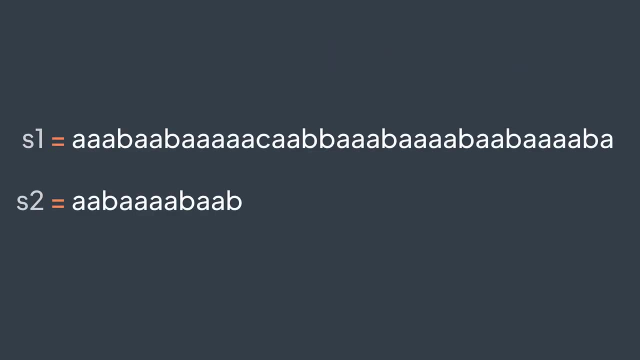 and increment i. as explained earlier, After filling the LPS array, we just return it. Now that we know how to generate the LPS array, we can use it for the KMP algorithm. Let's take this input, For example. the first step is to generate the LPS array of s2,. 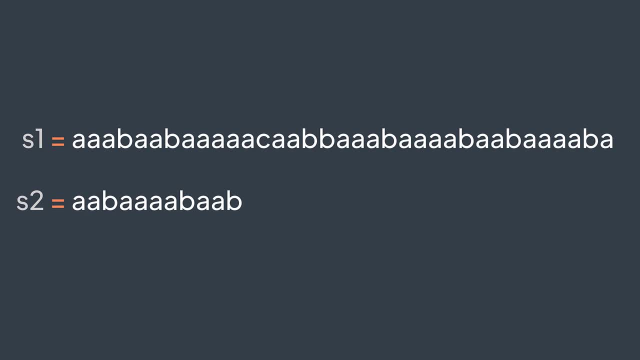 the string we're searching for, And s2 is the same string as the last example, So we get 01012223453.. Now let's start from the first character of both. They match, we continue, they match, we continue. now, s1 of i and s2 of j don't match, And the part that matches a, its LPS is a is length is one, So we 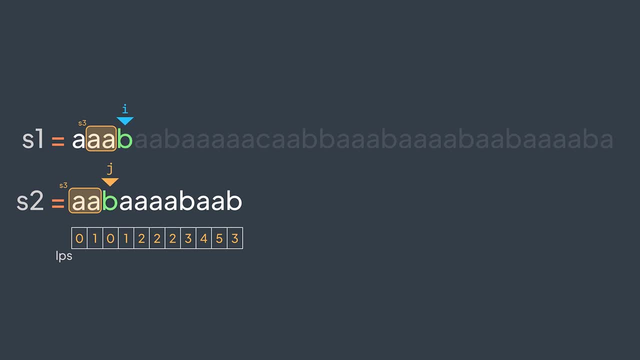 take j to one Now. they match next iteration. they match next iteration. they match next iteration, they match at next iteration. they don't match. j is five. So the part that matches a baa is LPS is a, his length is two. we take j to two. Note that here we're using quite the same logic as when. 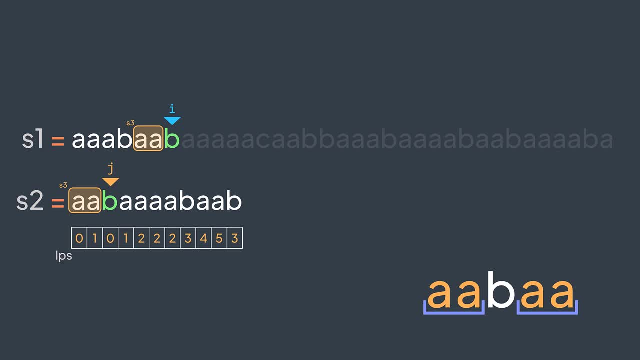 we're doing the array. For example, when characters match, we increment both i and j. when they don't and j is greater than zero, which are the LPS of the part that answer j minus one and we take j to its length. And when they don't match and j zero, we just increment our. to start. 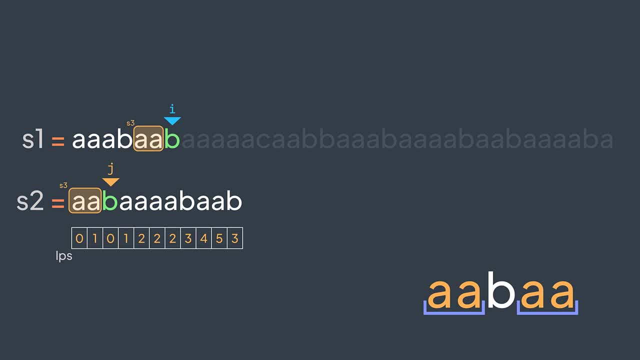 again from the next position of i Also, you can notice that we are able to get the length of the LPS directly from the array. we're doing it in all of one. we can say that we're able to do what we wanted to do since the beginning of the video: searching without taking back i to avoid losing. 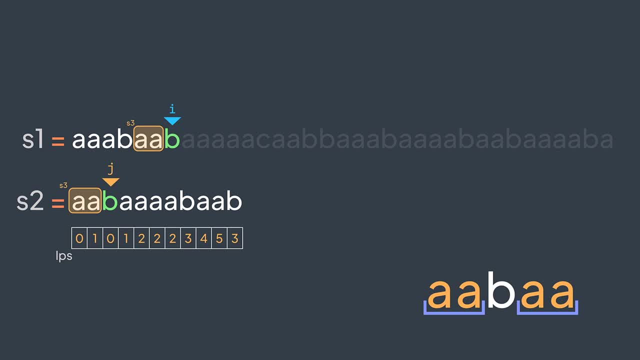 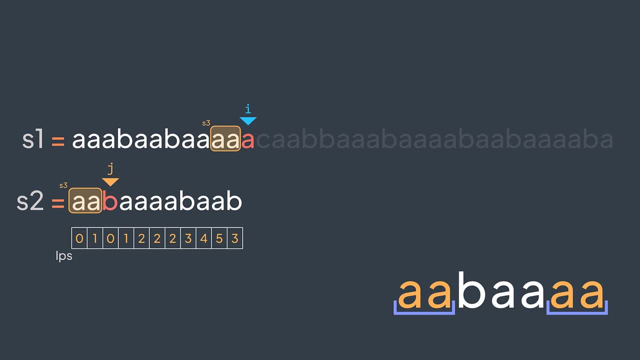 we take j to two. He also. they don't match the part that matches is the one that answer j minus one, which is a. its LPS is a host. length is one. we take j to two Here also. they don't match the. part that matches is the one that answer j minus one, which is a. its LPS is a host, length is one. we take j to two Here. also, they don't match the part that matches is the one that answer j minus one, which is a. its LPS is a host, length is one. we take j to two Here. also, they don't match the part that. 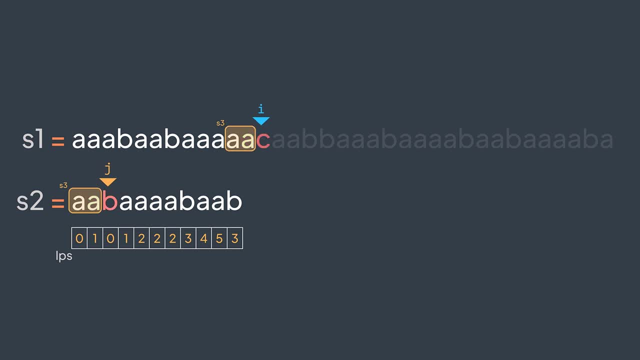 matches is a. this length is one. we take j to one. Here they match legend ration. they don't match The lps of the power. that matches is a is length is one we take j to one, He. they don't match again the LPS of, as the empty string, x length is zero. we take j to zero, They don't. 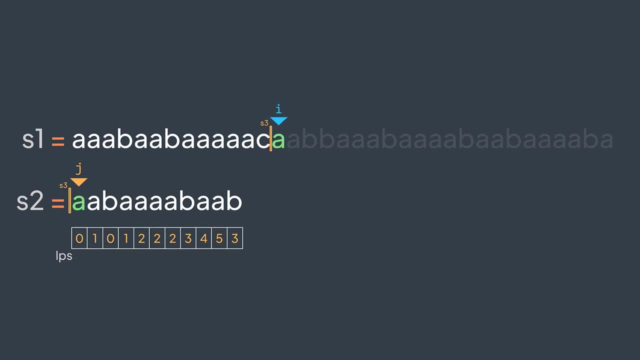 match again And g zero. we just increment I to start again. We have no choice. Is a match ass ration? they match this iteration. they match Next iteration. they don't match the pot that matches is a, b. its lps is the empty string. the length is zero. we take j to zero. Here again, they don't. 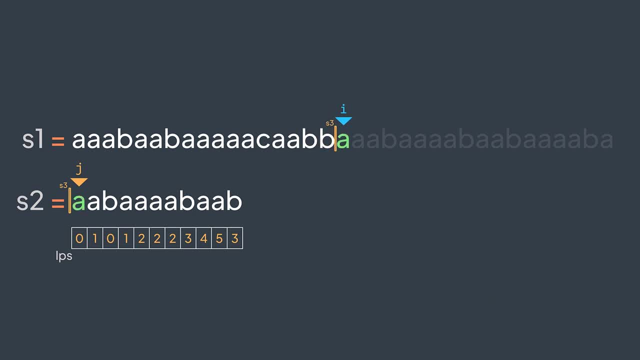 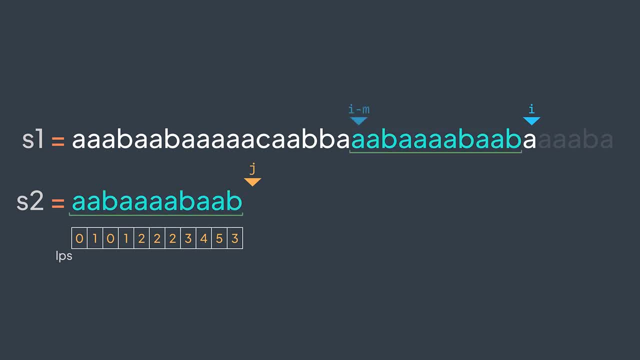 able to find s2 and s1, we turn i minus m, which is the starting position of s2 and s1, which is what we're searching for In code. we put the length of s1 and s2 in an arm respectively, And 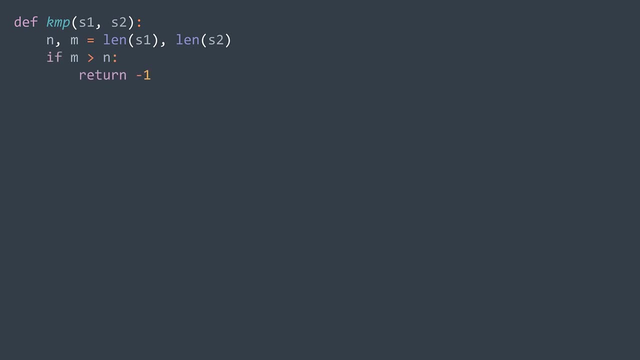 now we have some early exit conditions. If s2 is longer than s1, then we cannot find it in s1. Obviously we don't clear turn minus one. minus one means that we didn't find it Else if, as one in s2 have the same length, if they're equal, we're turned zero. 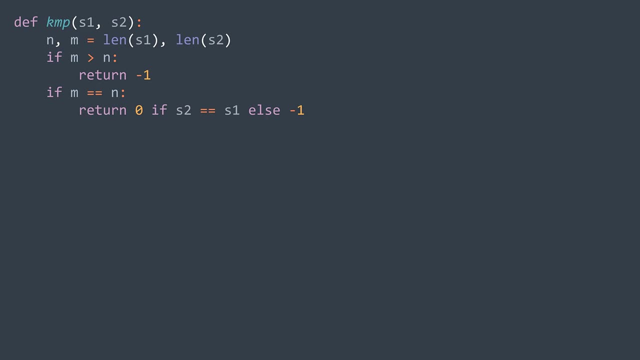 the index of the final first character, because it starts from there, And minus one if they're not equal, because if they have the same length, the only way to find s2 and s1 is by starting from the index zero and all characters match Else. if s2 is the empty string, we darkly return. 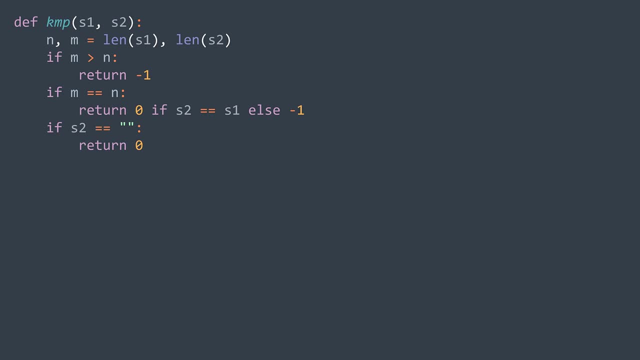 zero, because the empty string is a substring of any string. Now we can start. first of all, we saw that we do some pre processing to generate the LPS array of s2, we just call the function we made all you get LPS. Now that we have the array we put, I enjoy the first character. 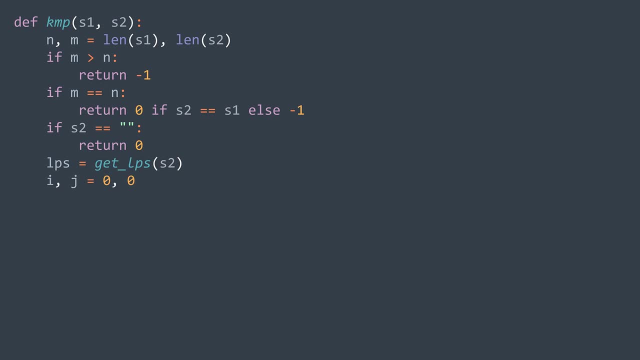 of s1 and s2 respectively 00. And we start looping. the loop stops when we reach the end of either s1 or s2.. Reaching the end of s2 means that we found it in s1, and reaching the end of s1 without the end of s2 means that the search was unsuccessful. Now we have. 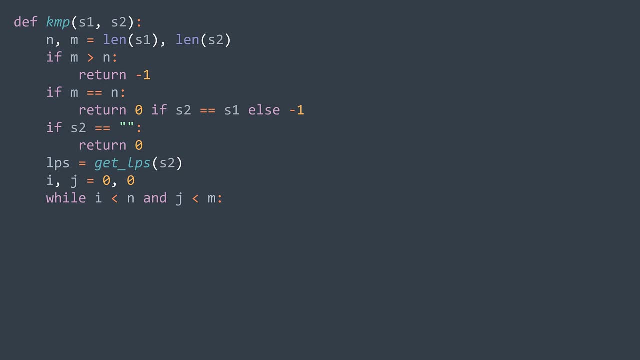 the same three cases as when filling the LPS array, but without assigning to an array because we aren't filling any array. If s1 of i and s2 of j are equal, we just increment both indices: we increment i and we increment j to move to the next pair of characters. Else, if they're not equal in j. 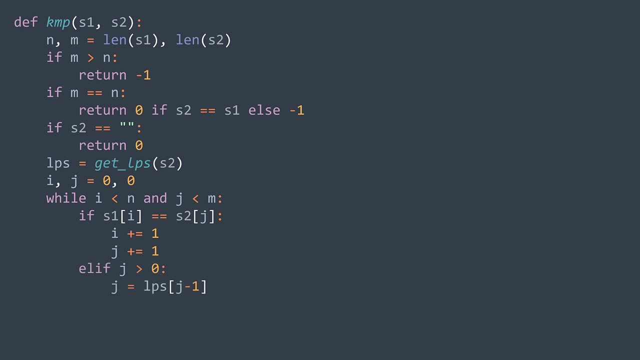 is greater than zero. we sell that. we take j to the length of the LPS of the part that matches the one that ends on j minus one, and its length is an LPS of j minus one. This is why we assign LPS of j minus one to j Else. if they don't match in j zero, then we 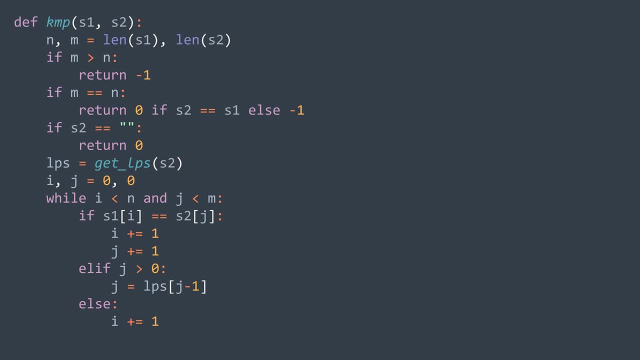 can't find s2 by starting or pressing from I, Because even the first character doesn't match. so we just increment i to start again from the next position. The second case, when we take j to LPS, of j minus one, is what we've. 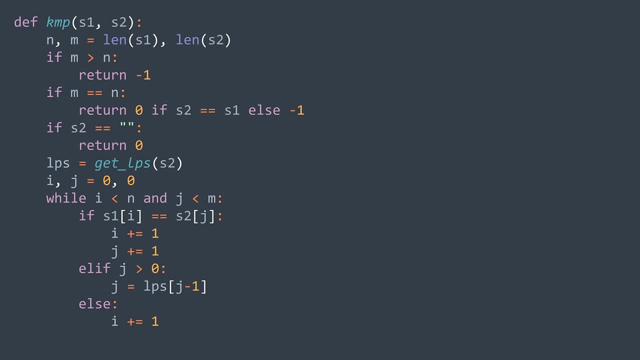 been explaining in the beginning of the video. It's a really important point that you need to understand. It's what gives us the ability to not take back. i We saw that from the LPS array. we can darkly know how many characters we can skip. This is why we take j to it. 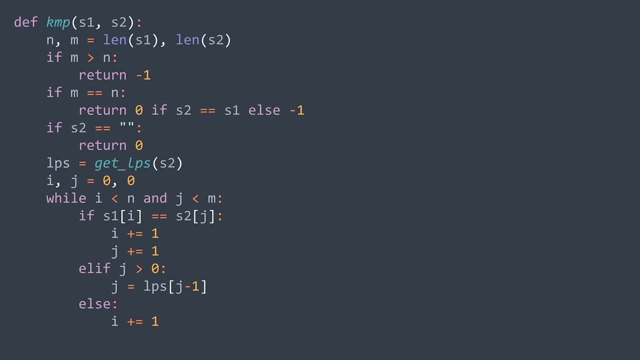 j in reality represents the first index from where we should continue comparing. If we take j to the second index, then we return minus one because it means that we didn't find it Else. if we found it, we return i minus m. i represents where we found the end. 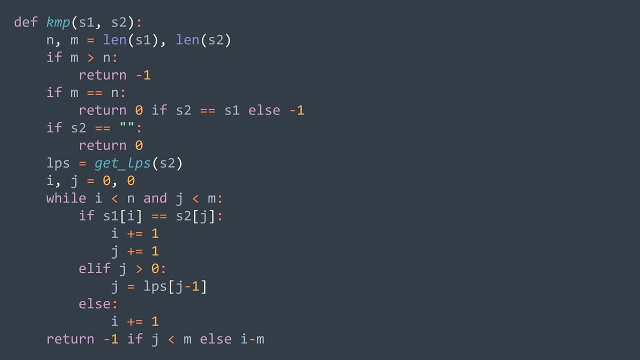 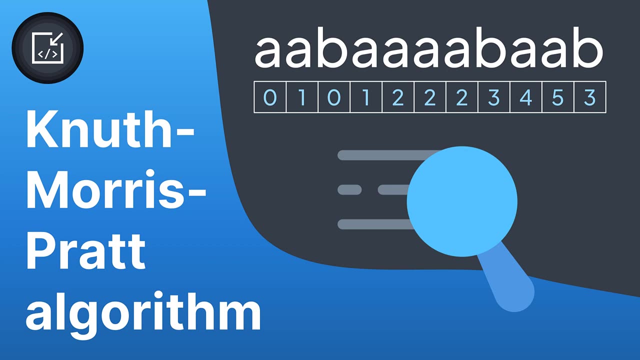 of s2 and minus m to go back to the starting index, because we want the index where s2 starts in s1.. And that's how the KMP algorithm works, An interesting string searching algorithm that takes advantage of the longest proper prefix. that is also a suffix of the part that 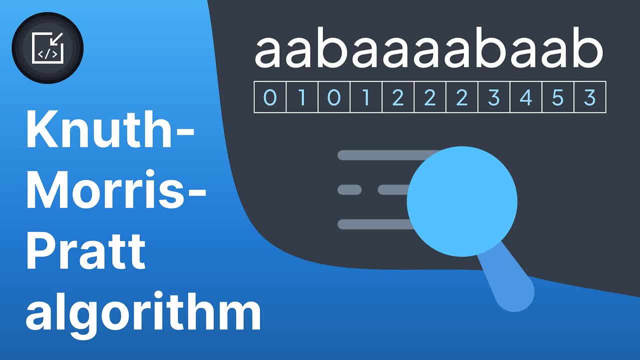 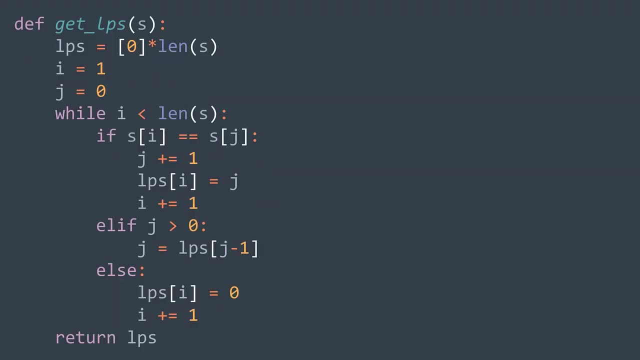 matched to be able to scale. Okay, now we know how the algorithm works, But what about its time complexity? For the time complexity, let's first start by analyzing the get LPS function. we want to generate the LPS array of a string of M characters. creating the array costs then for the loop. 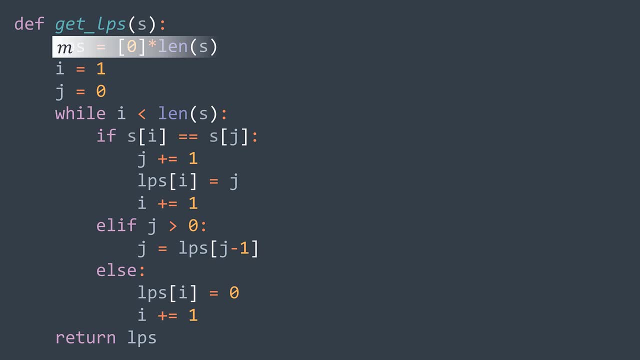 we're traversing the M characters with an index i, So we may think that the loop will do M iterations, But you can notice that i isn't getting incremented, that each iteration, so we may have more than M iterations. Because of that, we may think that in the worst case each value of i requires 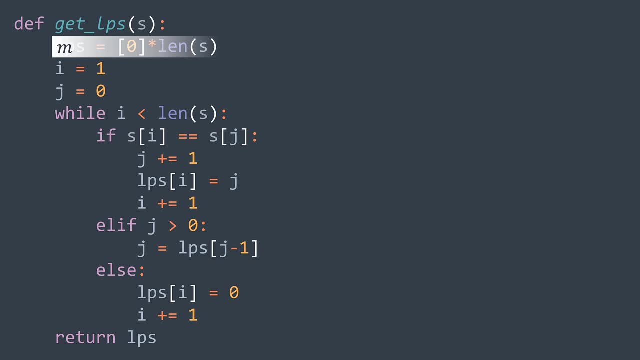 off M iterations before it gets increased, which would result in an off M squared time complexity. But no, let me explain. The second case is the one where i doesn't increase and to occur, j has to be greater than zero. And to have j greater than zero, it must have been incremented. 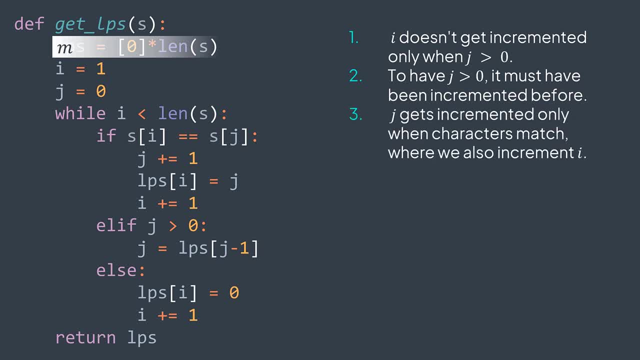 before incremented only one characters match where we also increment I. we did use that. we can't have the second case without incrementing I. We also know that in the second case J can only decrease when we assign LPS of J minus one to it, because LPS of J minus one. 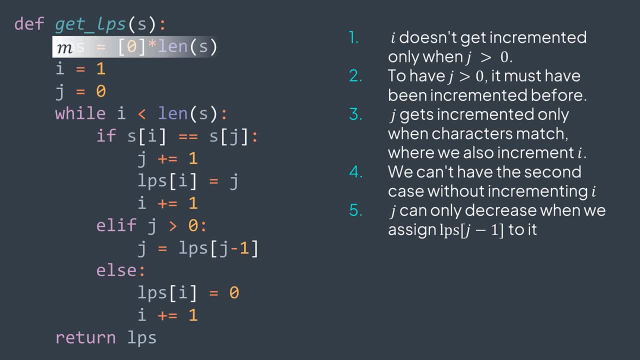 is always smaller than J From these five statements. we did use that because I gets incremented m times before the loop stops. it means that the number of iterations were the second case occurrences at most. m In total we have am iterations where I gets. 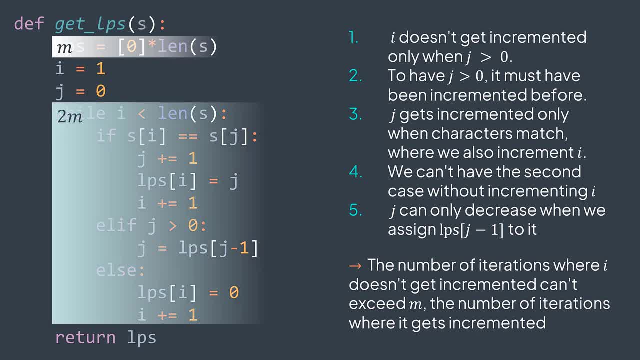 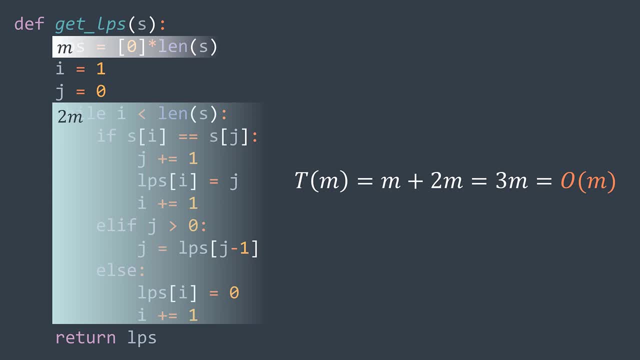 incremented and am iterations where it doesn't. we'll get out most two am iterations for the loop Plus for array creation. we get three m, which gives an O of m time complexity for the get LPS function where m is the length of the string passes. an argument Now for 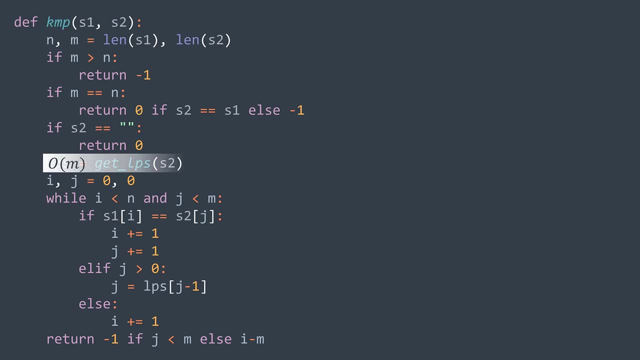 the KMP function, we have O of m for calling the get LPS function. then for the loop, we may think that in the worst case we do any durations. And because n is greater than m, because cases where n is smaller than, 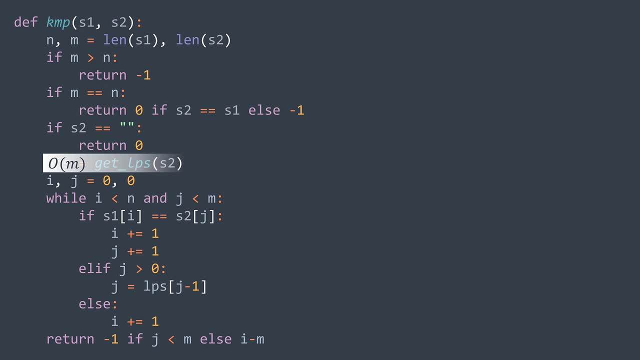 or equal to m are handled by early exit cases. But here also we have a case where I doesn't get incremented in the second case, to be precise. So we may have more than any creations. But same logic as for get LPS to form the second case: J must be greater than zero. In other 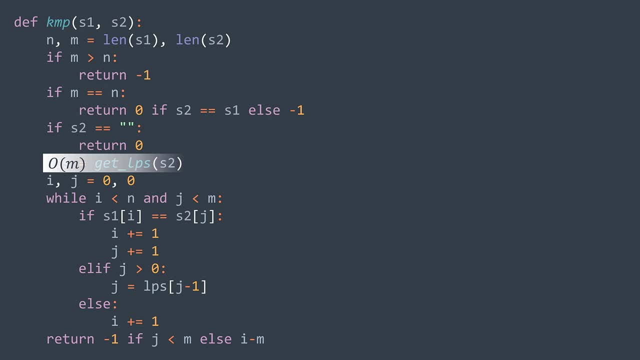 words, it must have been incremented before, which is not possible without also incrementing I, and is incremented n times during the process. So the number of iterations where it doesn't get incremented can't exceed n In total. in the worst case we have any durations where is incremented and any durations where 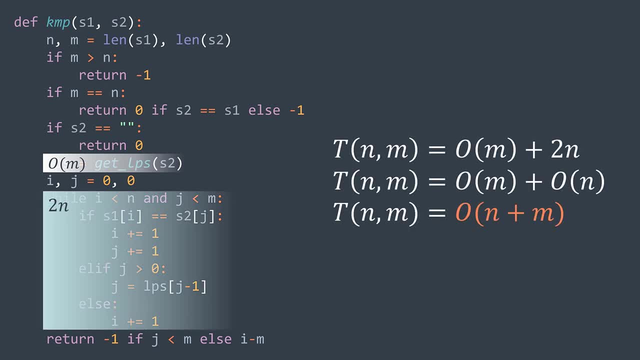 it doesn't. And plus n is two n which gets off n. So we have O of m for generating the LPS array of and for the loop we get an O of m plus m time complexity for the KMP algorithm And for the space complexity. it's O of m because of the LPS array. Know that, even if. 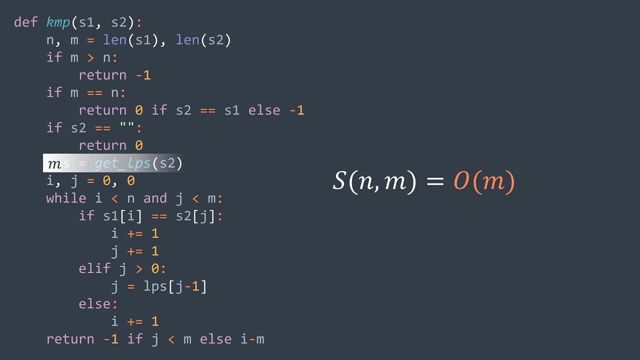 the KMP algorithm has an O of m plus m time complexity. it doesn't mean that it's always the best choice when it comes to string searching. It depends on the length of the two strings, overlapping substrings and all the factors. This is why there exists situations where 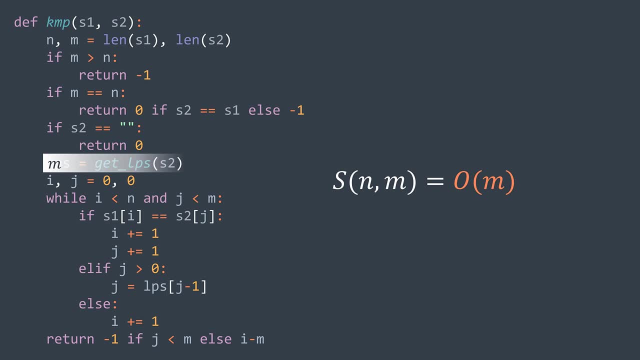 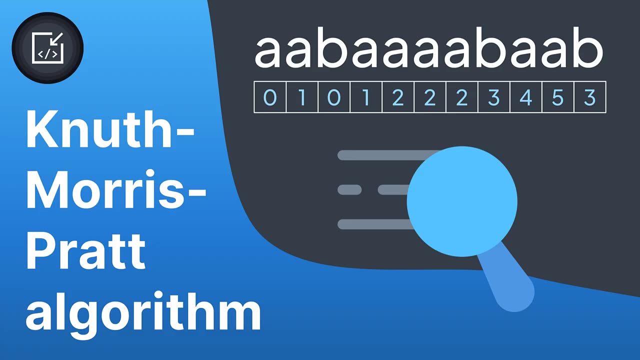 we would use another string search and algorithms like Robin Karp and buy more. We use the end of this video. I hope that I've been able to explain to you the KMP algorithm. Give me your feedback in comments, like and subscribe to the channel and see you in the next one.